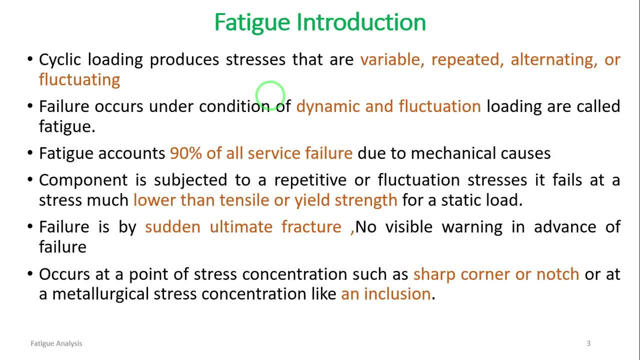 than the tensile or ill scale. therefore we have to consider this fatigue while designing, then this failure is a very catastrophic type of failure or sudden ultimate fractures. we can say: and it not. it does not do any prior warning or in advance warning in the failure and occurs at a point of stress concentration such as sharp. 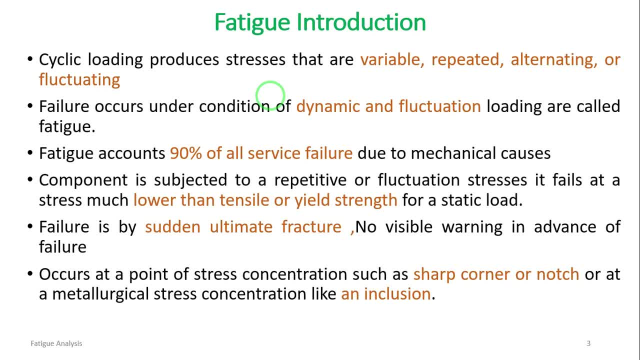 corners or not, or at a metallurgical stress concentration like an inclusion. so where there is a sharp corners or abrupt change in cross-section or poor surface finish or we have notches in the component, in this case in that place or point we have a stress concentration and this stress concentration leads to a 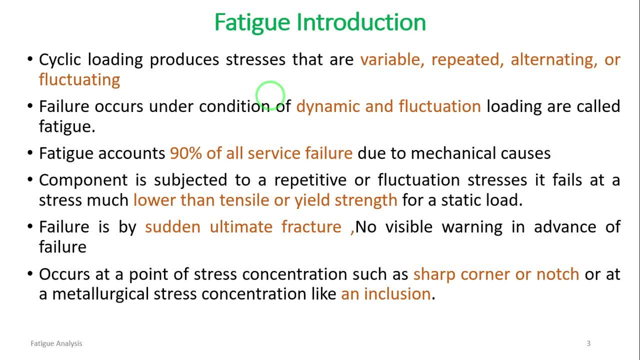 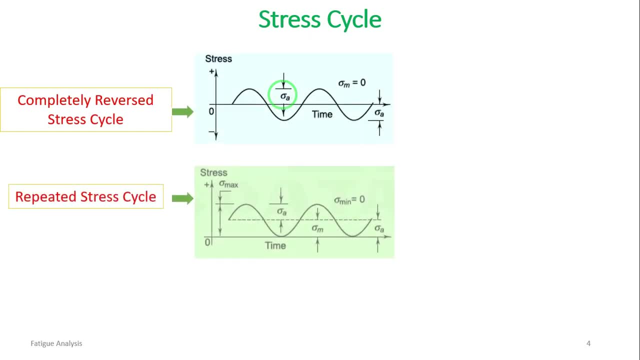 crack, generation, initiation or propagation, and then the component is going to fail after the number of cycles. so this is a basic idea of the failure, of the fatigue, this failure. then we have stress cycles. basically we have three type of stress cycles. the first is completely reverse stress cycle. second is repeated. 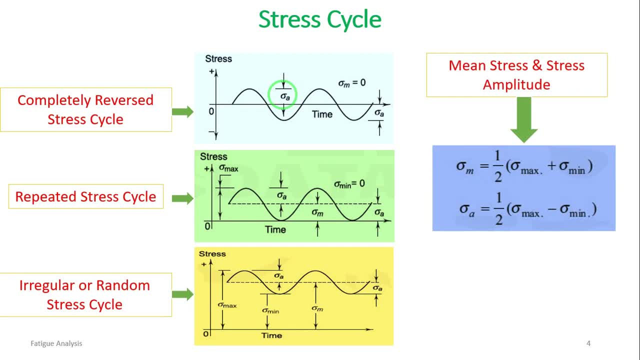 stress cycle. and third is irregular or random stress cycle. so here there are some terms like mean stress or stress amplitude. the mean stress is Sigma M, which is given by maximum stress plus minimum stress by 2, and stress amplitude is given by maximum stress minus minimum stress by 2. 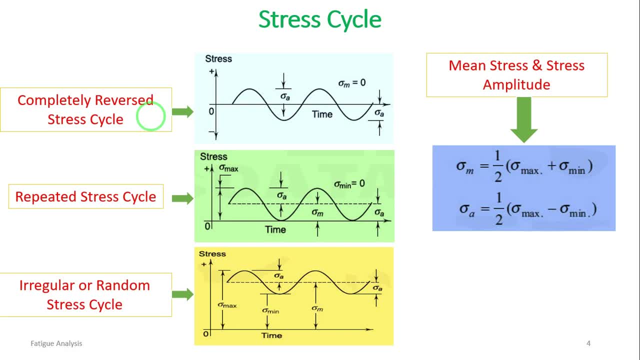 the first case, that is completely reverse stress cycle. we have loading which is completely reverse and the load are come, are equal in magnitude but opposite in directions. so consider example of candelabra and we are going to apply load in downward direction, which is of 100 kilometer and the same 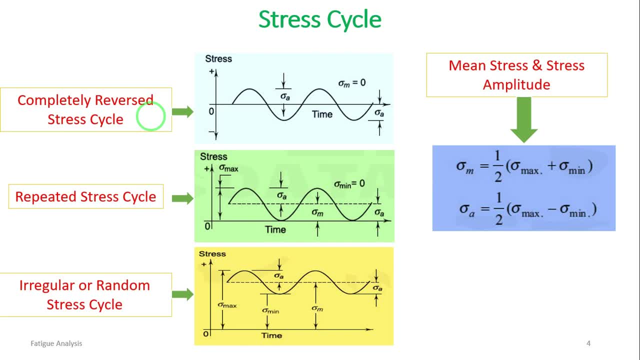 force which is applied in the upward direction, having the magnitude is 100 kilometer. so we have the loading of equal magnitude, but in opposite directions. so in the first case- that is completely first case- the mean stress is zero because the maximum stress and minimum stress are. 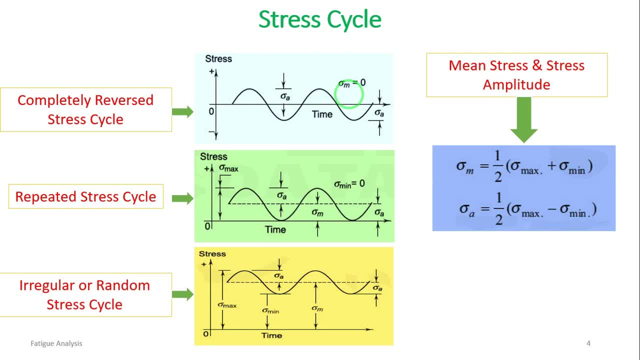 equal in magnitude and opposite directions. that is also known as tensile stresses and compressive stresses. so here the mean stress is zero and your stress amplitude, which is equal to your maximum stress and minimum stress. then, second type of cycle: in this case your minimum stress is zero and your mean stress value, which is equal to your maximum stresses. 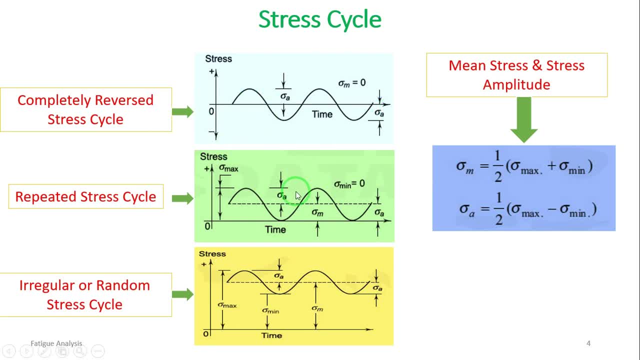 right and mean stress value and stress amplitude and maximum stress have the same values. and last one is irregular or random stress cycle. in this case we don't have a particular stress values. they are random in nature, they are time dependent and it is very difficult to predict the type of nature of the loading. so this is all about this video and if you 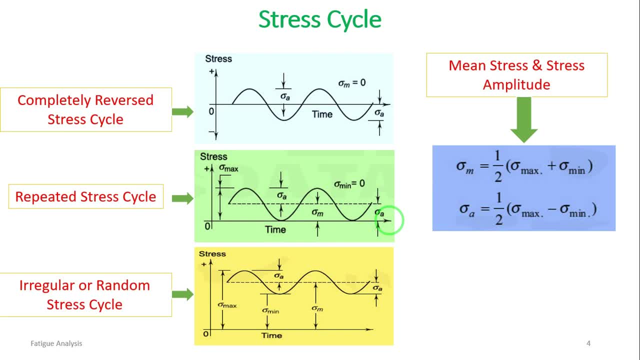 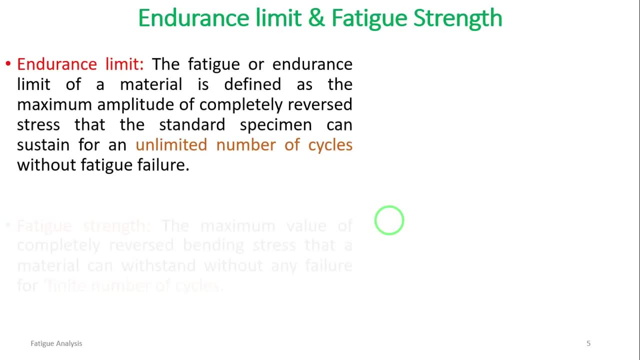 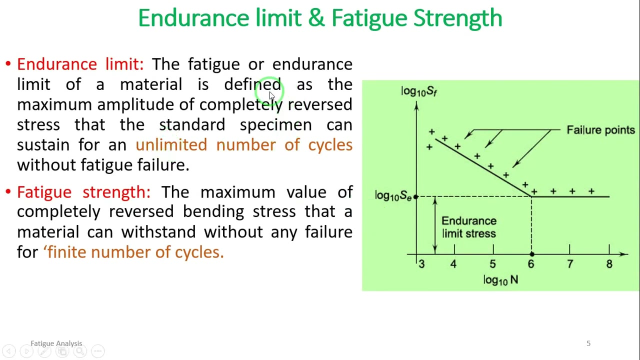 want to know more about stress cycles, and we generally have these cycles in the nature or components. so next, these two terms are very important- this fatigue analysis, so endurance limit. so here the fatigue or endurance limit of a material is defined as the maximum amplitude of completely reversed stress that a standard specimen can sustain for an unlimited number. 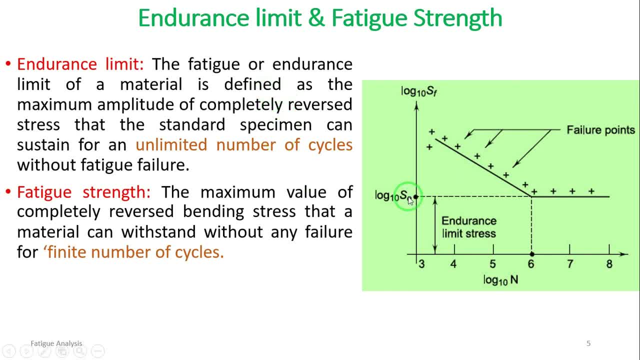 of cycles without fatigue failure. so here in this graph you will see this log, 10 scale paper, and on the horizontal axis you will find stress cycles and vertical axis you will find a stress amplitude. and here this SE is nothing but your endurance limit and the stress value if less than this endurance. 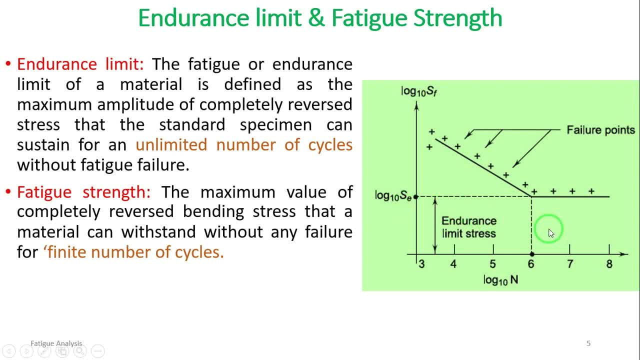 limit, then your component is not going to fail and it has an infinite number of cycles. right, that is nothing but your endurance limit. and here you can see that when there is an endurance limit, value over the graph is a straight line and life will be component for this endurance limit is infinite number of cycles. so this: 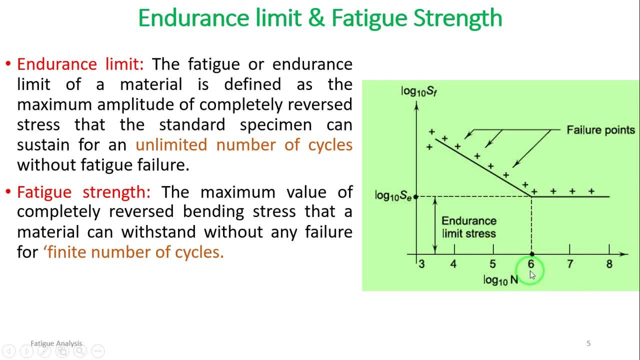 is your endurance limit, and here for structure steel, you can see the your endurance limit value is occurred at the endoscopic cycles. so this is a endurance limit, and here you value. next is fatigue strain, so maximum value of completely reverse bending stress that a material can withstand without any failure for infinite number. 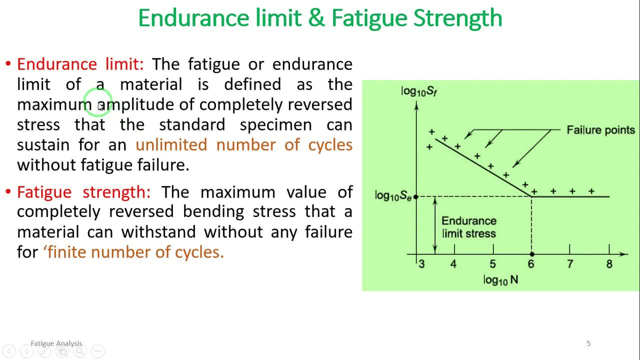 of cycles. so this endosymmet is for infinite number of cycles and this fatigue strain is for finite number of cycles. and here these cycles below this endosymmet is known as your finite number of cycles, and here the failure occurs. in this region, the 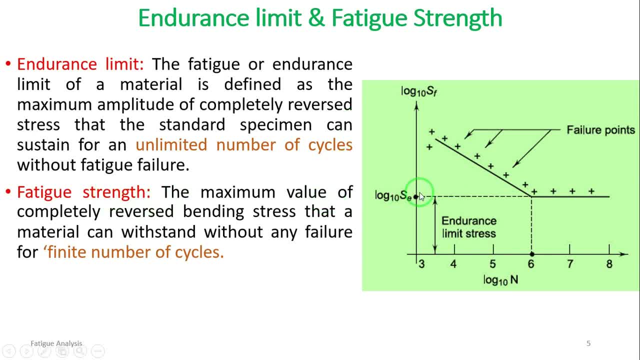 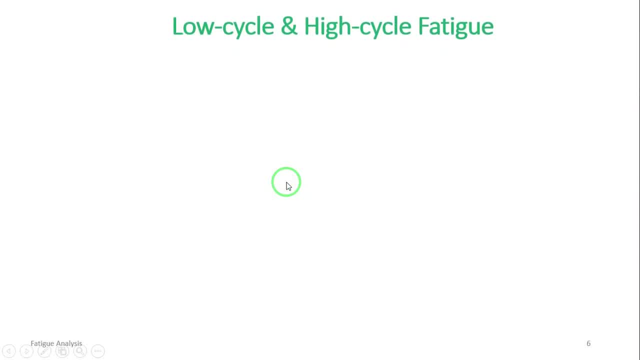 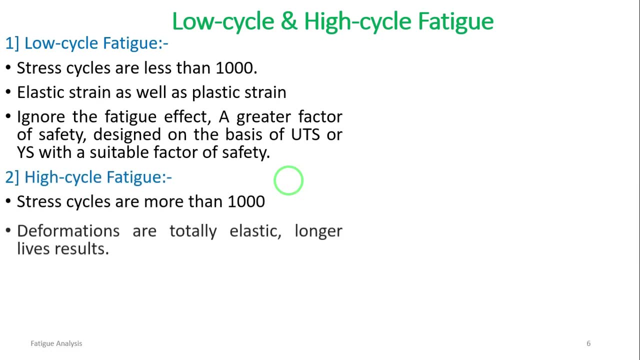 strength we can have here is fatigue strain above this endosymmet and fatigue your component is going to fail for this finite number of cycles. so next slide, we're going to explain what is mean by low cycle fatigue and high cycle fatigue. so first is low cycle fatigue. so here in low cycle fatigue, the stress cycles are 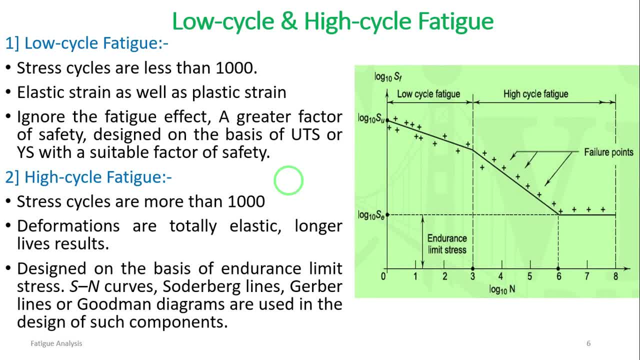 less than 1000. so whenever, if you find Keep life having the stress cycle releases in 1000, then it is known as blow cycle fatigue and in this case we- this component- going to experience both the reformation that is, elastic strain, as well as plastic soils and sometimes the 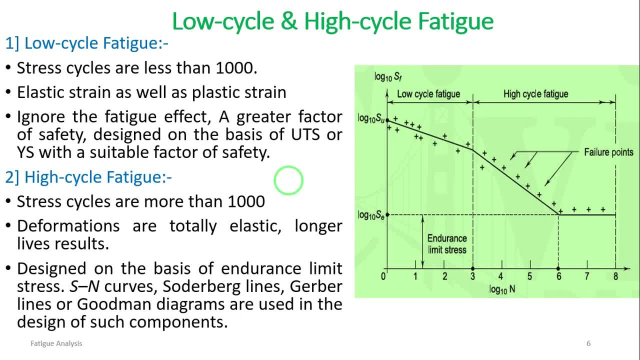 designer is going to ignore this fatigue effect and he has to consider greater factor of safety. and sometimes we have to design the component based on the ultimate instance strength or yield strength with suitable factor of safety. so it is when we have stress cycle less than 1000, and in this case the loading is or: 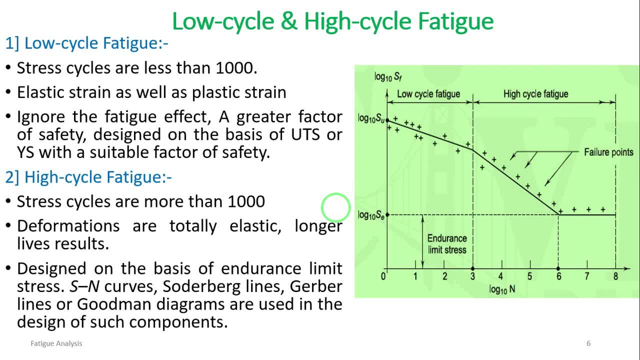 this type of application is having the lower high load applications. therefore, we have to sometimes we have to ignore this fatigue effect and we have to consider greater factor of safety. but in case of higher cycle fatigue, whenever there is this cycles more than 1000 and this deformation is only of elastic nature and and the load conditions or 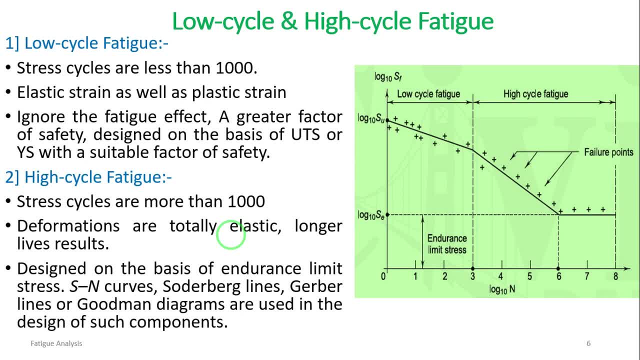 load applications, very uh, small in this case, which is known as high cycle fatigue, and this, uh, in this case, the design of component is based on endurance limit- stress, because for endurance limit we have infinite number of cycles- uh, like a component. and there is another terms like sn curves. 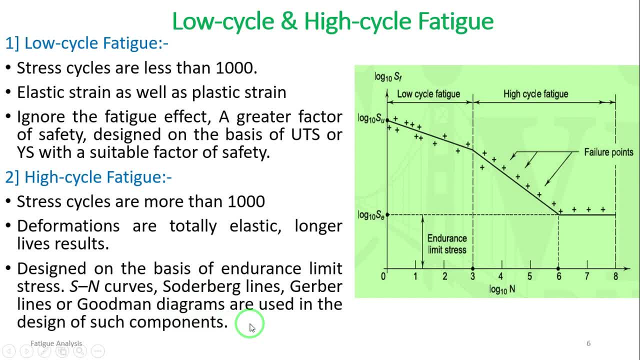 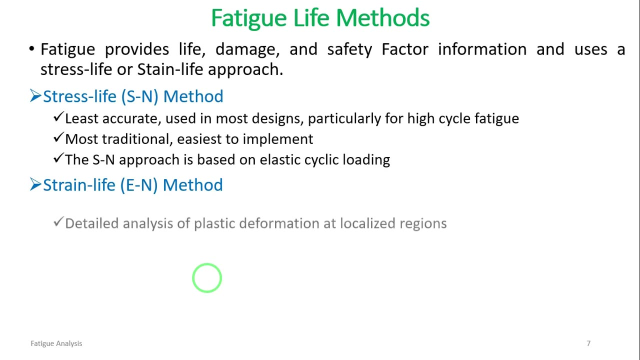 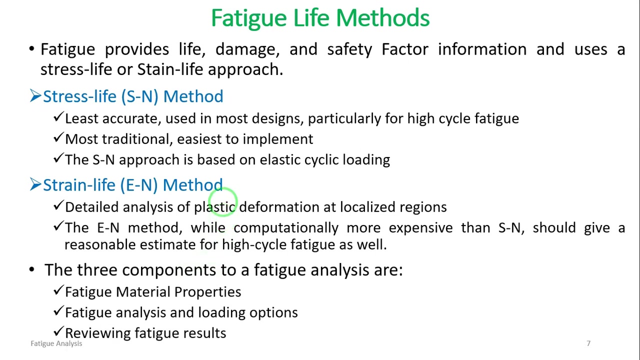 shoulder. bug lines, verbal lines or goodman diagram are used in a design for of such a components. so generally we consider this high cycle fatigue for the analysis and we use this other terms to calculate the design components. next is fatigue life methods. so we have different terms here, like life fatigue and factor of safety. so by using the answer 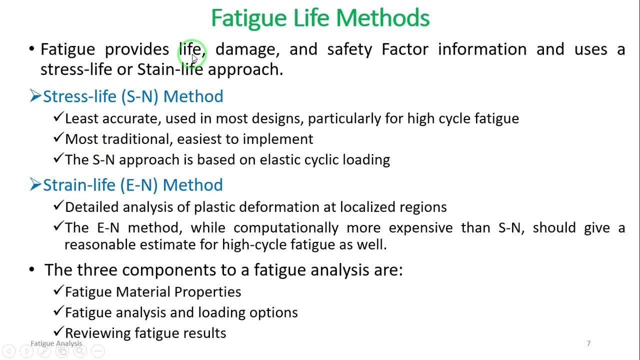 weapons. we can able to find this life in cycle, hour or days. there are number of options. we have to find the life of the component, then damage. so here damage is something that gives information about your component is going to fail or not. if the damage value is less than one, then your component. 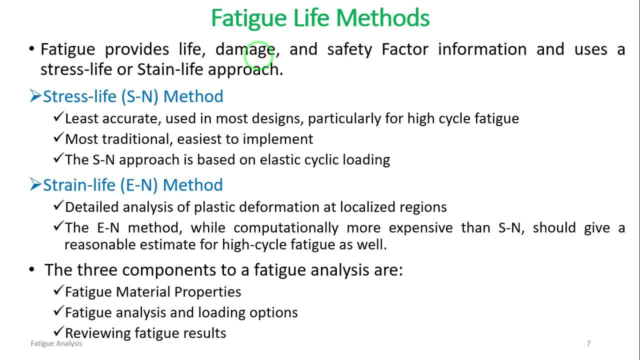 is not going to fail. if damage value is greater than one, then definitely your component is going to fail. so it is something- the ratio of design life upon minimum life- that is calculated using the given loading conditions and factor of safety. so all this information can be can be. 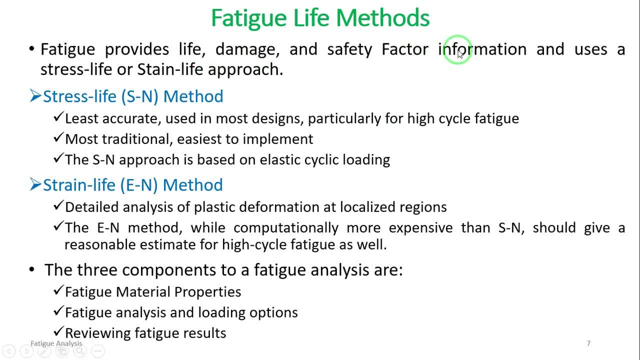 calculated by using the answer web bench and we have two approaches to solve any component for the fatigue analysis: that is stress life, the sn method, and second is strain life, that is en method. so let's understand what is the stress life or sn method. so this method is a very initial method, or we can say traditional one method and it is least accurate. 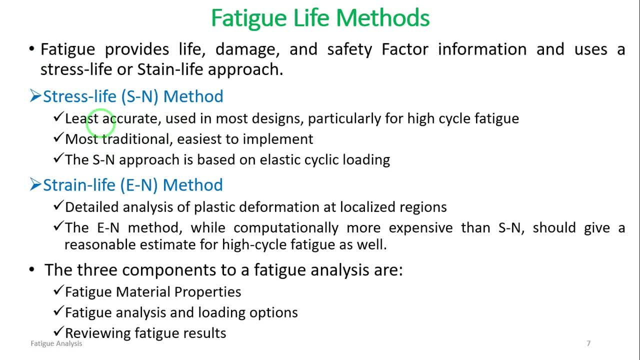 but it is very easy to implement. therefore, this you will use in many design processes, and it is particularly for high cycle fatigue. right, and this sn approach is purely based on elastic cyclic loading, so here we are not going to consider any plastic cyclic loading or plastic strains, right? so these are the some other dangers of sn methods. next, is this strain life or en? 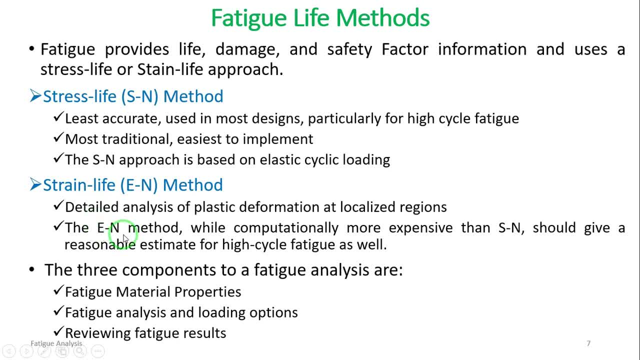 method. so this is: this method is you used to determine the plastic deformation at localized regions, and it is totally based on this strain instead of elastic. and then this en method or strain life method is more expensive than sn method and but it is give more reasonable estimation of results. we can say if we are 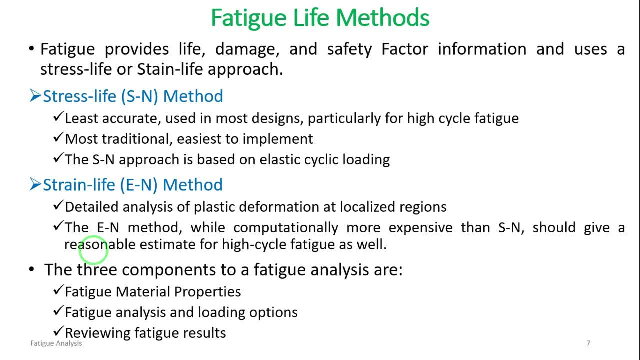 going to bear the computational cost, then we can use the strain life method instead of stress life. but in our case or example, we are going to use this case like method. there are three component to a analysis. the first is fatigue material properties. so we required generally alternating mean. 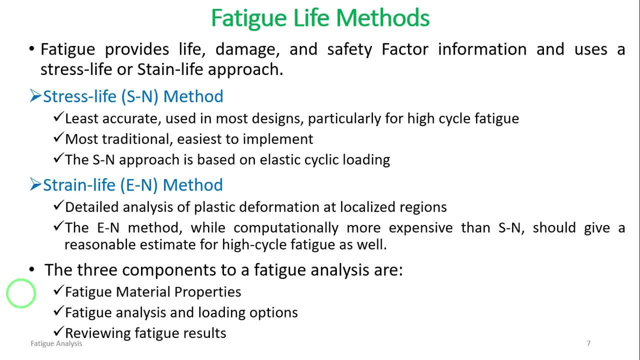 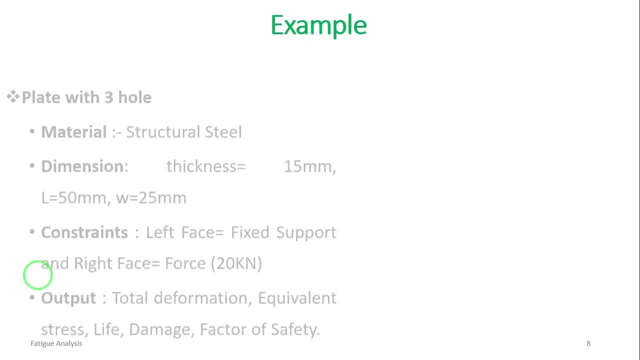 stress or strain, life method, properties or curves required in the property menu of this fatigue analysis, then fatigue analysis and loading options. so here we have to do the analysis setting, like loading conditions or boundary conditions. then we have to do the fitting results. so next slide is about example that we are going to solve using a silver. 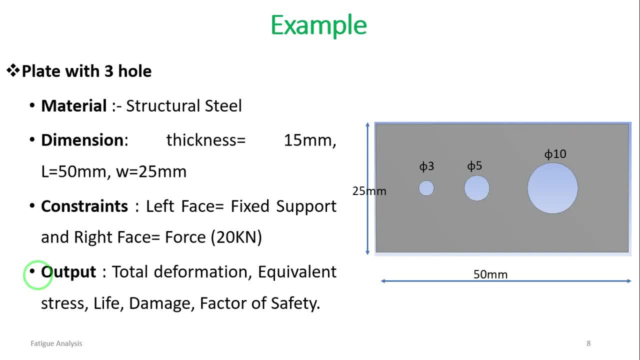 bench. so here we have plate with three hole and the material of the plate is structure steel. so here is dimension of the plate is so 50 is the length of the plate, 25 is the weight of the plate and 15 is the thickness of the plate and we have three hole of diameter. 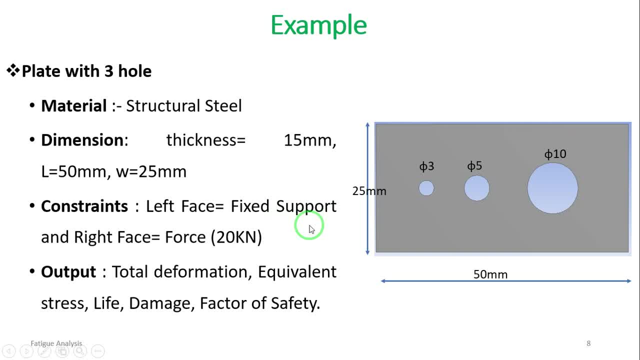 3, 5, 10 respectively. so the left face of this plate is having the fixed support and the right face of the plate In the force of 20 kilometer. and here we have some. we required some output, that is, total deformation, equivalent stresses or one minus stresses, life of the component in cycle. then 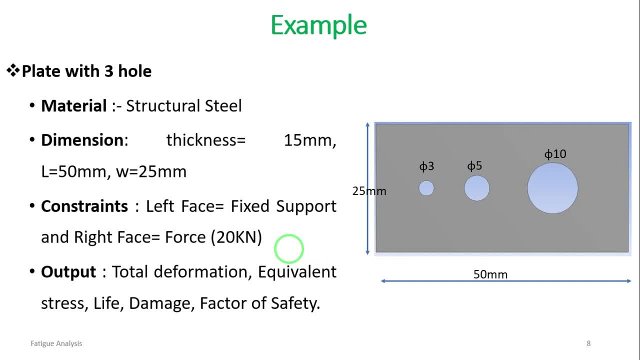 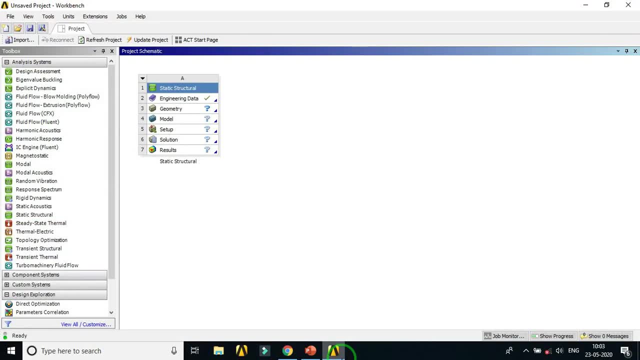 damage and factor safety. so this is the example we are going to solve in a silver bench. so let's start with a silver bench. so here I have open this, a silver bench, and we have created this static structural analysis system in post schematic. so there is a we don't have. 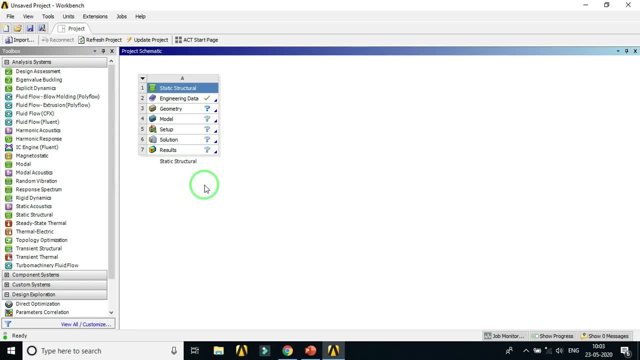 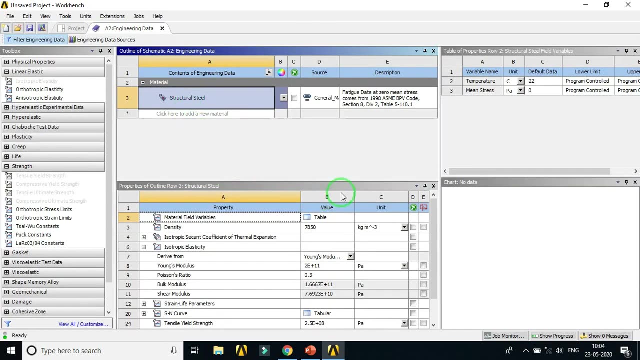 another analysis system for separate analysis system for fatigue analysis. we have to use this static structural analysis in that we have fatigue tool. based on that fatigue tool, we are going to find these results. so you have first click on this engineering data. so we have to see what type of property we require for fatigue analysis. so ensure that. 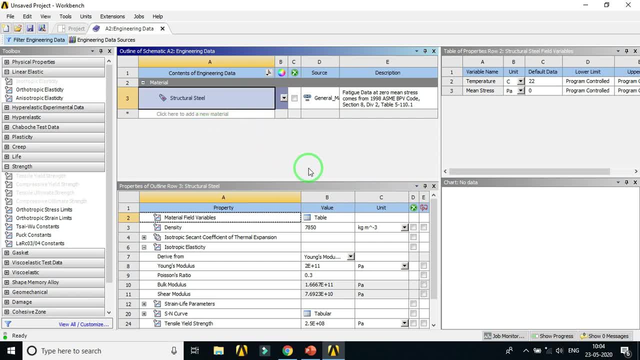 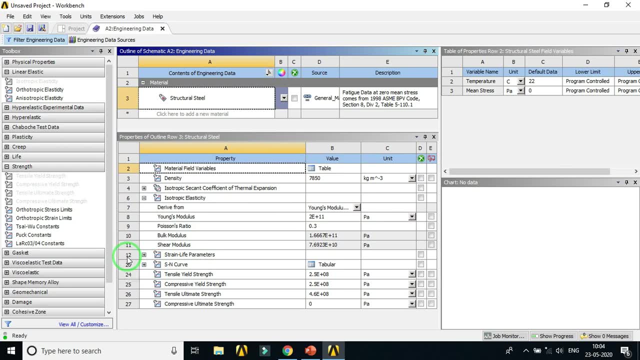 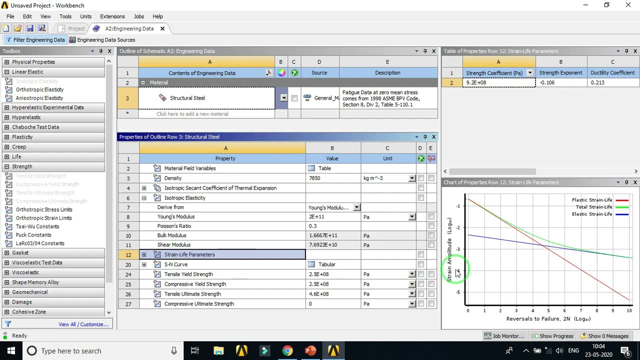 this structural steel tab is selected and the property of outline row is visible, and here, the row number 12, you will find the strain life parameter. so when you click on the strain like parameter, you will get some chart here and there is a plastic strain like, total strain like 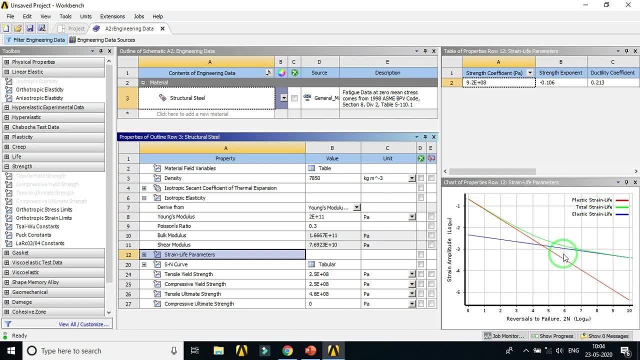 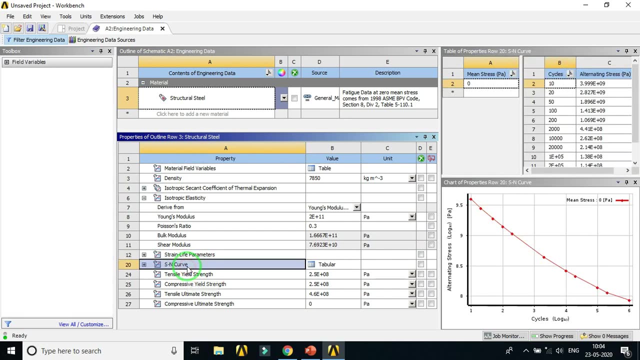 and elastic strain, like. so these three curves showing this, similar parameters, and this is for this structural steel like material. so we have different these parameters or curves for different materials. then next is sn curves, the stress strain life curve here. so, based on this alternating stress and cycles, we have this graph and here, for vertical axis, we have alternating stress and for. 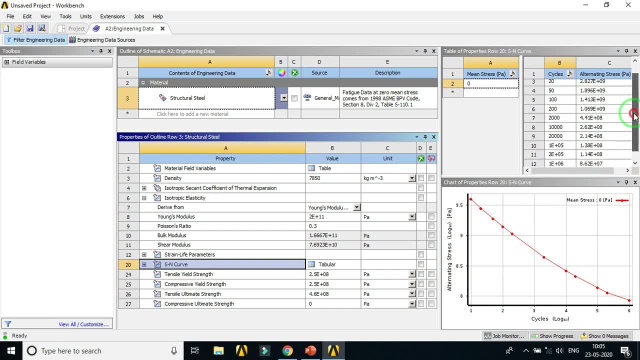 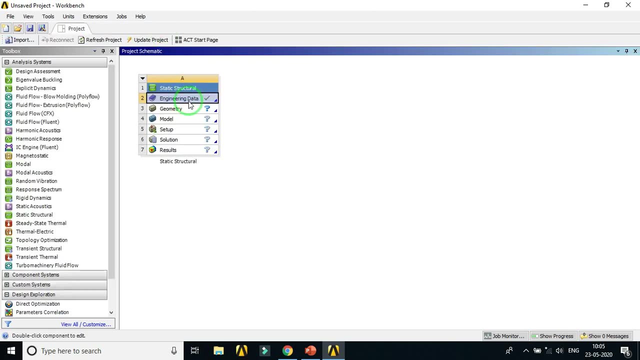 horizontal. we have cycles. based on this experimental data, we have created this graph. it is stored in this axis library. so this is main two parameters or property required for the fatigue analysis. so close this engineering data and we have to generate this geometry in the design model. so 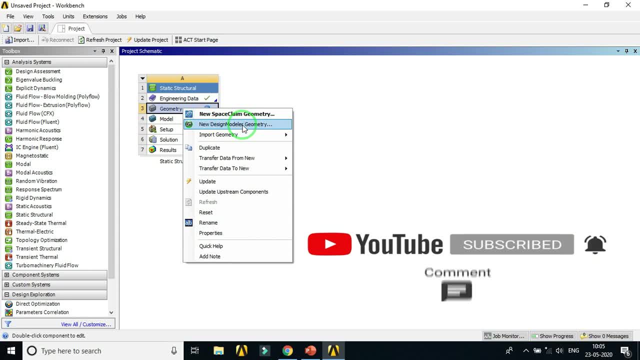 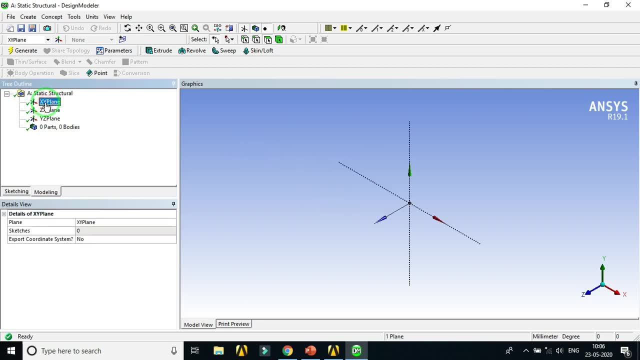 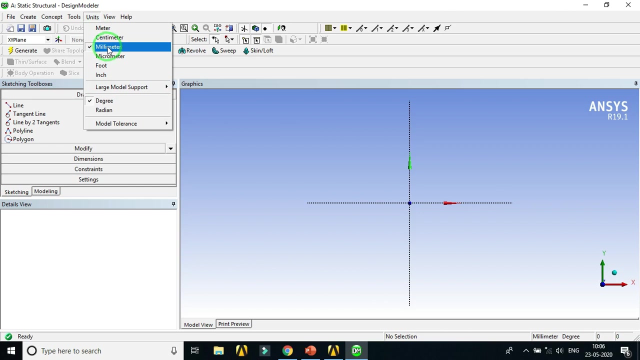 i click on geometry and select new design model geometry. so this is design model. click on this x bar plane and i click and click on this look at to orient the plane. then click on this sketching and here, before that, click on these units and ensure that the units in millimeter, then select. 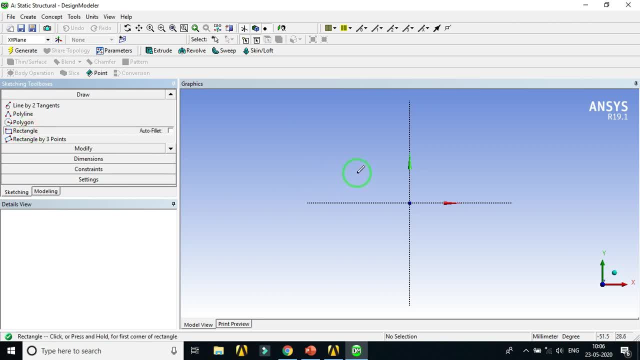 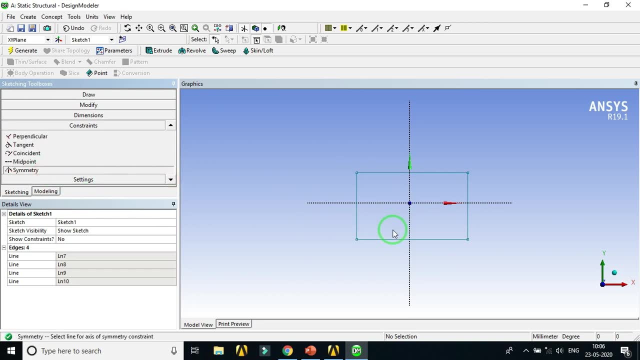 rectangular tool from the draw toolbox and create a rectangle. then apply some constraint here, that is, symmetry constraint, then select vertical axis, then select two sides of the rectangle, then again right click, select mute symmetry axis, again select horizontal axis and select this to set the rectangle. so here we have given the this symmetry. then we have to: 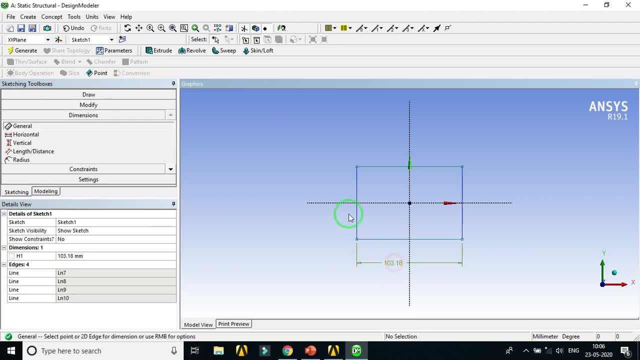 do some dimensions here. so this is uh 50 and this is 25. so go to the dsv and give dimensions here 50, then vertical it is 25 to 25.. so in this way we have created a rectangle. then we have to create uh, three circles. so 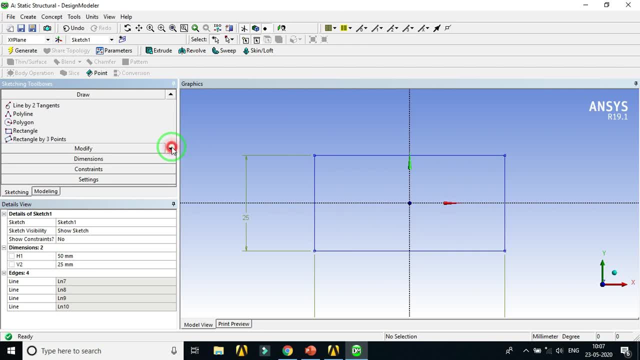 again click on this draw menu bar and select circle from the dot view box. create first circle, create second circle and create third circle. dimensions or diameter for the circles: this is the 3 mm, next is 5 mm and last one is 10 mm. so most of the dimensions are random. 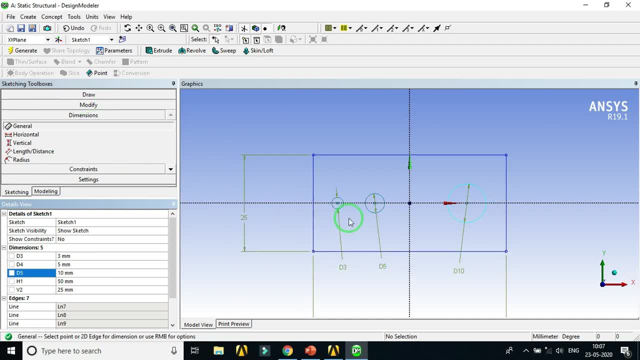 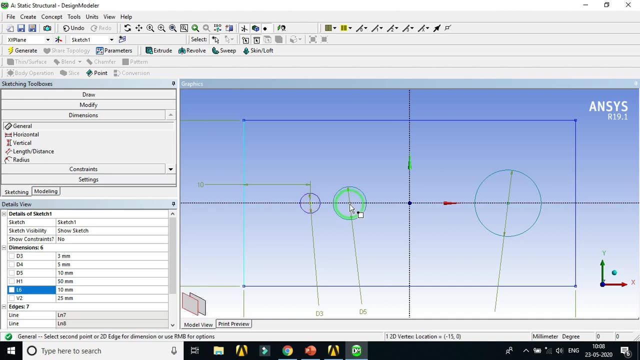 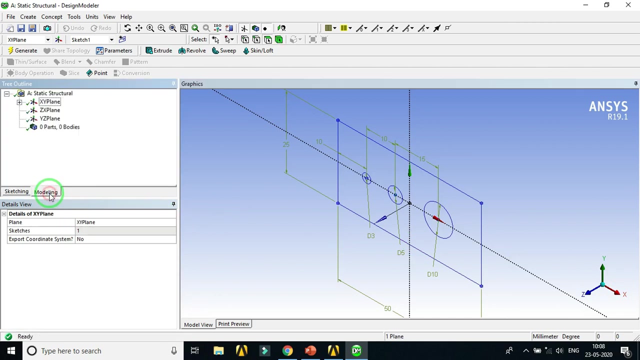 dimensions. so here we have to do another dimensions like the distance from center to the vertical edge aside, it is 10 mm, then again, then again between this second and third circle is hooked in. so in this way we have created the sketch. then click on the isoball, select this modeling mode and use extrude command. 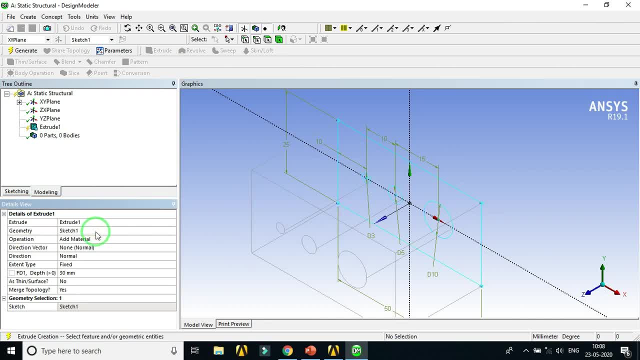 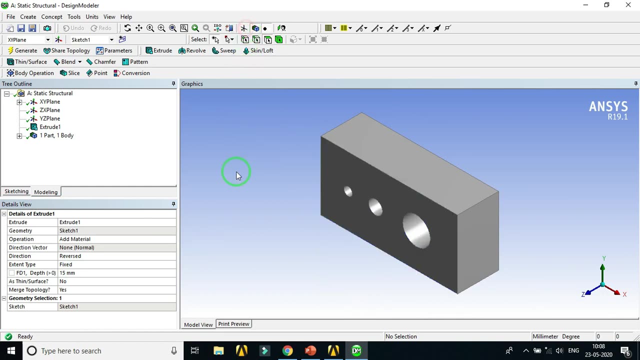 so it is asking for geometry. so it is, geometry apply and the direction is reverse and depth is 15, so thickness of the plate is 15, and click on generate and hide the sketch. so here, our plate with three holes is ready. so close this design model. 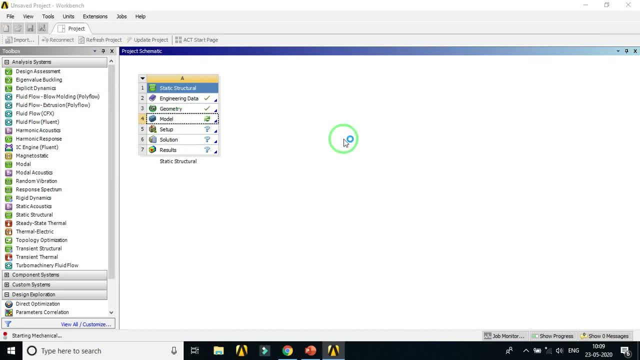 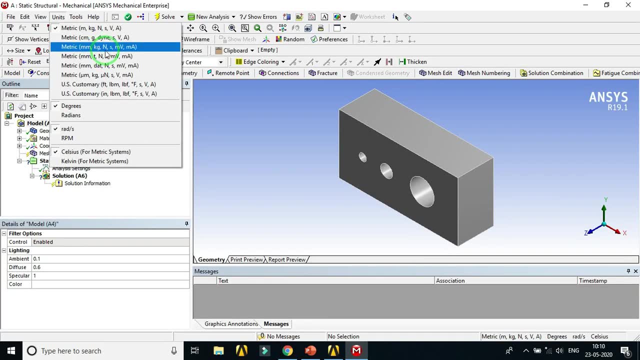 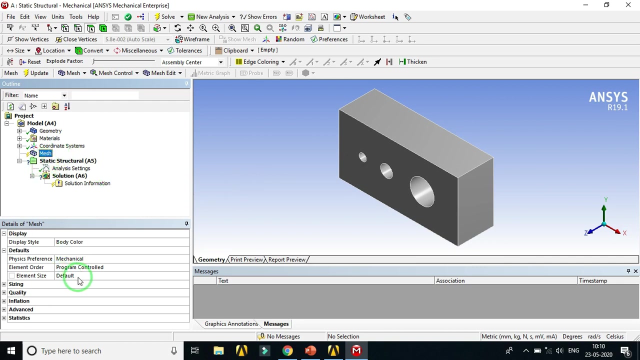 so double click on model to view the analysis settings. here is a. it should be in mm, so select the third options: mm. kg. newton. then we have to create a mesh for this. i am going to change. i am going to change this element size is suppose to mm and generate the mesh. so i am. 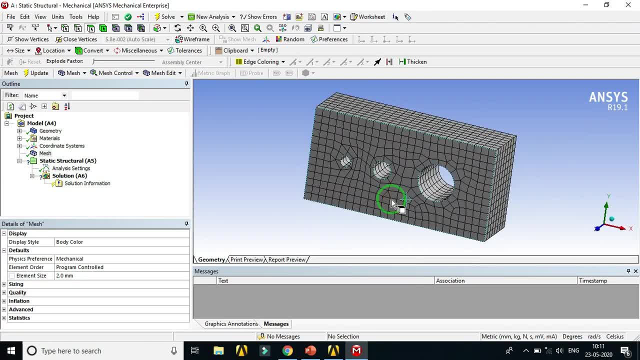 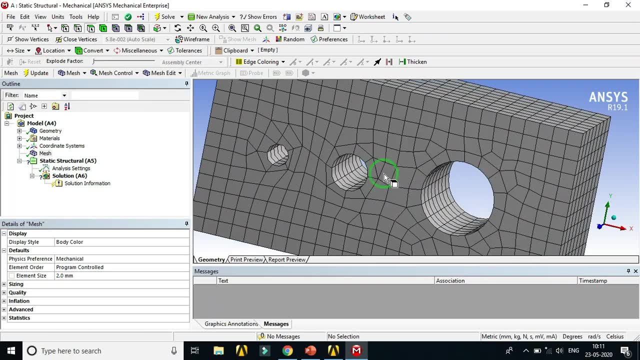 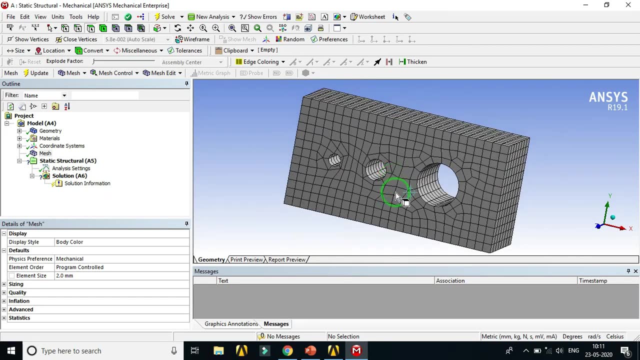 going to change the size of the mesh. so in this way our mesh is much better and there are some elements, but it is acceptable because we have different holes here. therefore, to create a uniform machine, we have to create a washer on the hole and we have to perform. 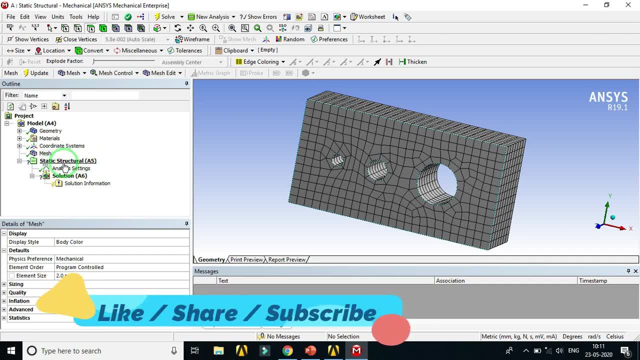 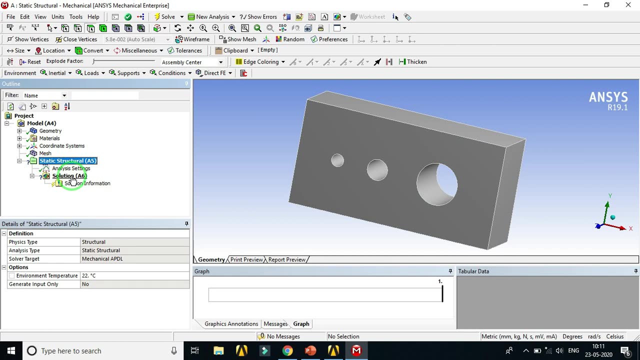 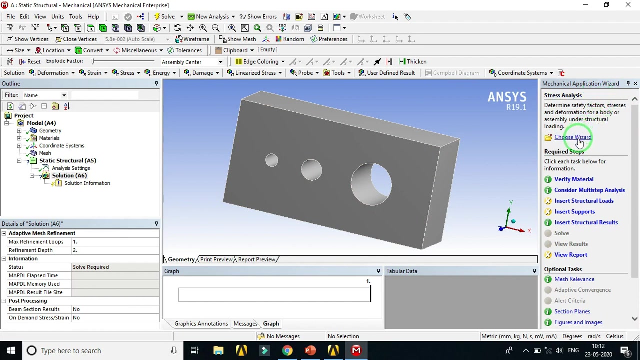 the mesh. again, we have two different methods. first is using the mesh and then we have to create a mesh, and then we have to create a mesh and then we have to create a mesh and then screen vogs such that all the blocks are. we can usng the staticity. 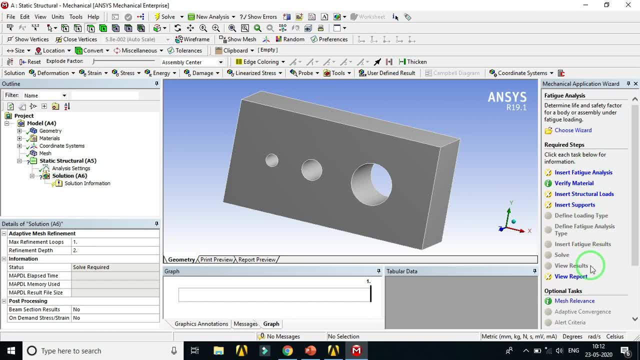 analysis. When you click on this fatigue analysis, then all the parameters regarding this fatigue analysis will be shown below here. So, from the first to last, it will show you which parameter is completed or which is completed, and when you click on this parameter, then it will guide. 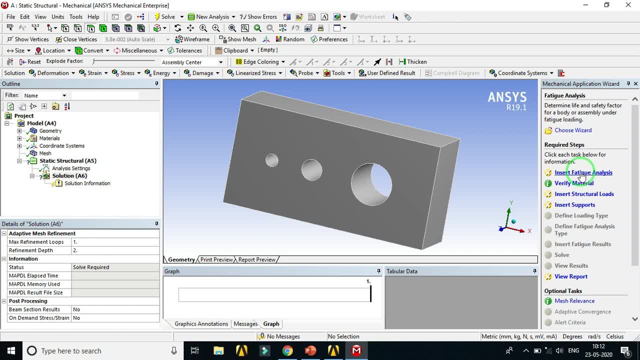 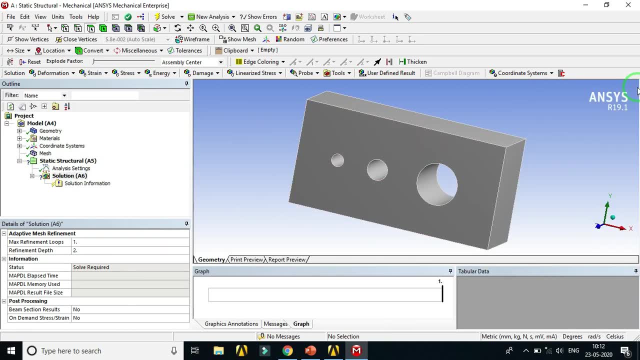 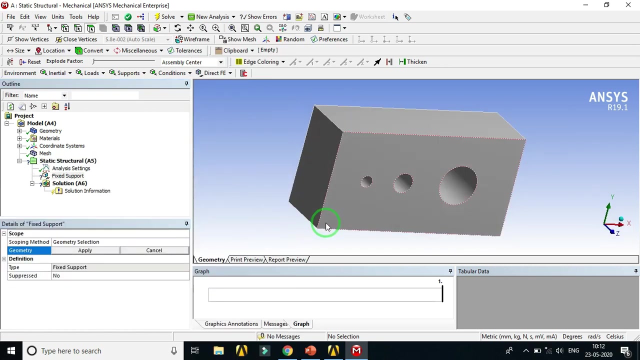 you how to perform this analysis. So instead of this, I am going to use this first method and close this window. Then here, click on the static structural, then right click on this insert, fix the port- Left face, left, left face. apply then again static structural loads. 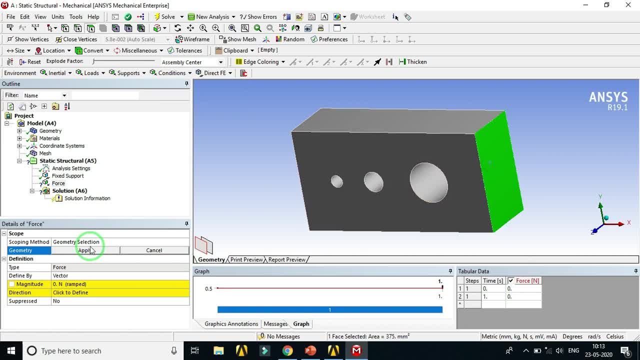 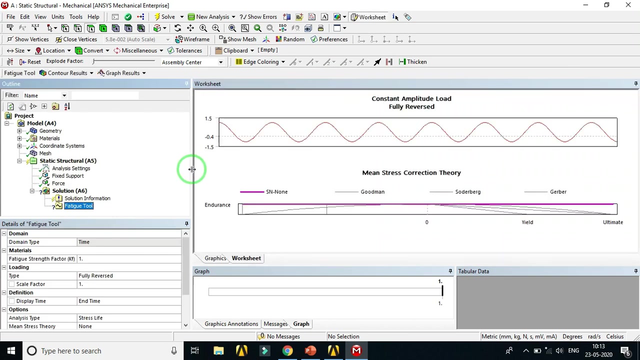 that is force on the right face. apply, defined by components along the right side of the plate: X axis, that is 20 kilo Newton. right then here, click on solution and insert tools, fatigue tools- right. So in the fatigue tools you will see this graph here, right click on this fatigue. 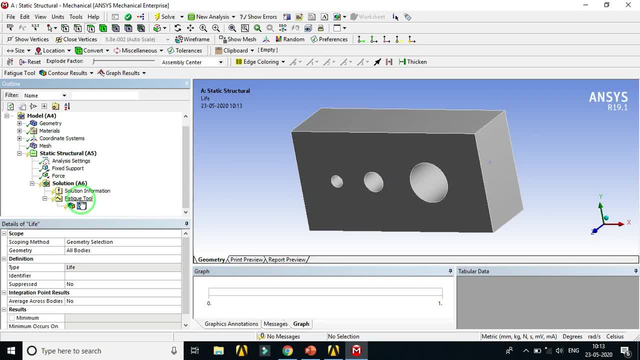 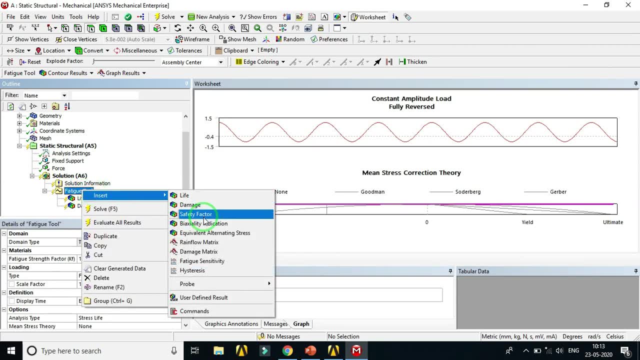 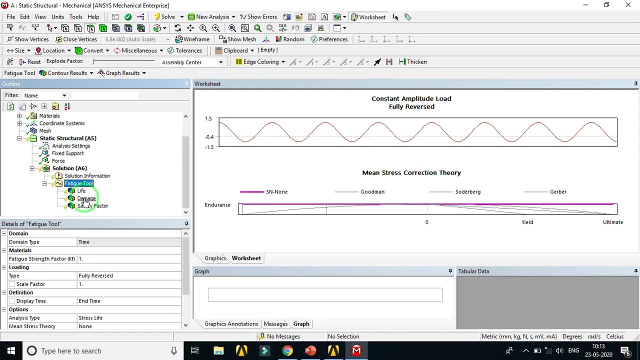 tool. insert versus life. and again right click on this fatigue tool, insert. Insert damage. again right click on this fatigue tool, insert this factor of safety. You can also insert, like equivalent adrenaline stress, but here we want to see these three values. therefore I have inserted it. Then click on this fatigue tool. you will find number of 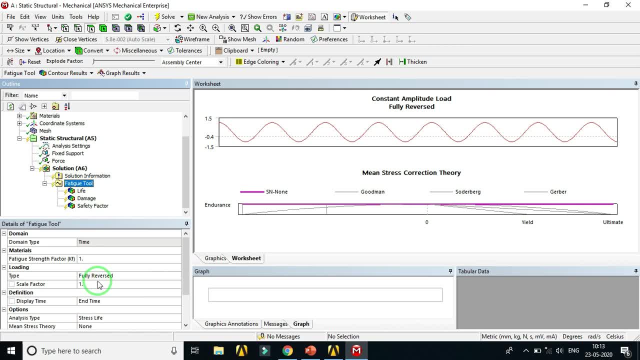 parameters there, So we will. I am going to extend this parameter one by one. So here details of fatigue tools. The first in the materials tab we have one setting is local control- is fatigue strain factor. So we have different factors available, like size factor or service finish. 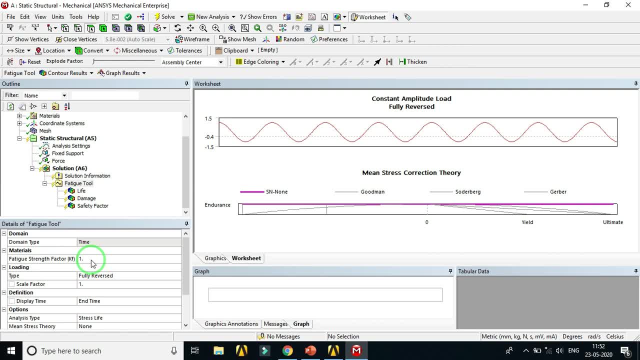 factor or many more. So if you have these values, you can use this here. So different values, one, and next is loading. So in the loading, in the types we have, different options are available, like fully reverse, zero base ratio, earning history data. So for fully reverse, 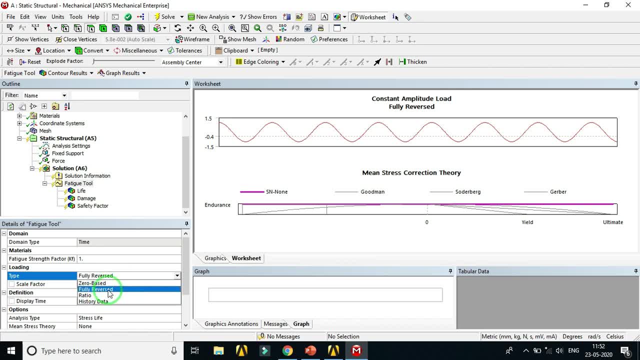 if you are loading having the fully reverse, that means the magnitude of the force is tensile and compressive, having the same magnitude. In this case we can use fully reverse. So this diagram will indicating the fully reverse type of loading, Here the maximum and minimum. 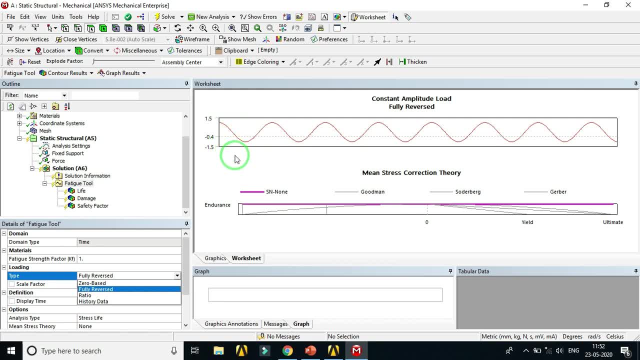 stress amplitude is equal, that is 1.5. and second option, that is zero base, it is a reverse, we can say, or repeated type of stress. we can say here: And if you have this type of stress and if you have this type of loading, we can use this type of options or this options. 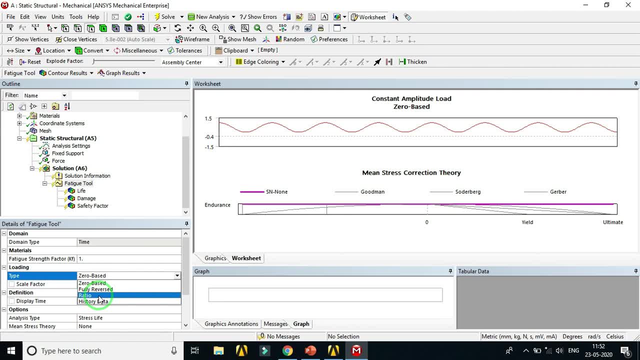 Then third is ratio. Instead of you have stresses value or loading value, if you have value ratio of the two applied forces, in that case we can use this ratio option. or if you have the loading value at different times and it has different values, then in that case we can. 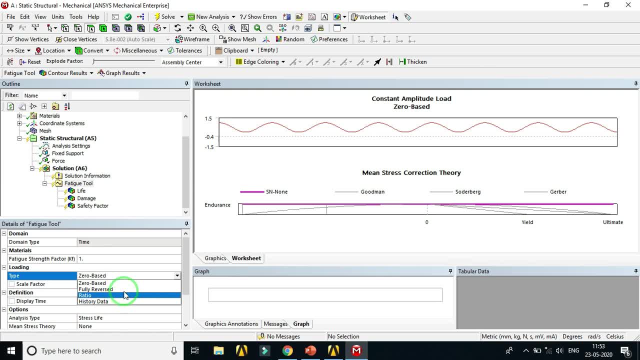 use this history data For the simulation. I am going to use this fully reverse. So here, from this, we can change the type of loading, Then scale factor. So it is nothing. but if you want to scale the amplitude of the load, then we can change it by from here. So the different value is 1. 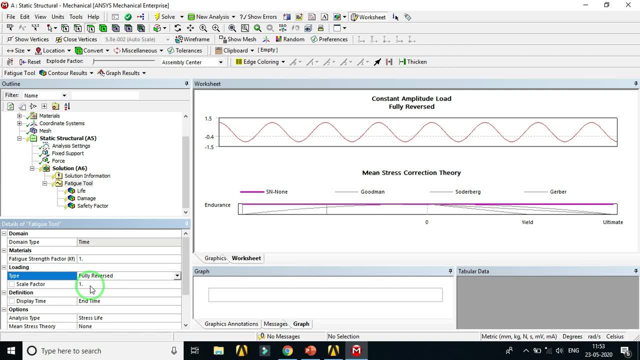 that means whatever value we are going to apply in the force condition or loading condition, it is same value is going to apply on the component. Then next is Here in options setting, analysis, set type. So here we have two different approaches, that is, stress life and strain life. As we already learned what is mean by stress life and what 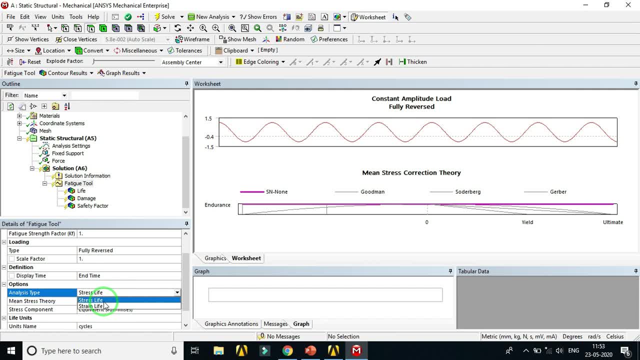 is mean by strain life. So for high fatigue or life we are going to use stress life, Then mean stress value. So practically, for completely reverse type of analysis or type of loading, we have zero mean stress but in practical it is not. We have mean stress value is zero. So by using this different methods, we can find the mean. 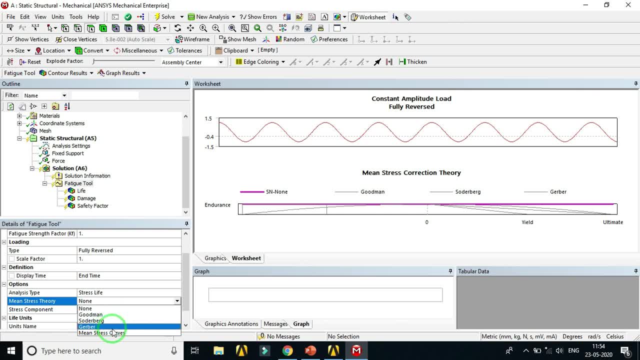 stress values. right, So goodman, featherberg, gerber and mean stress curves. These are different methods. by using this we can find the mean stress value After this. So last is unit names. So unit names. default setting is cycles. So from you can change. 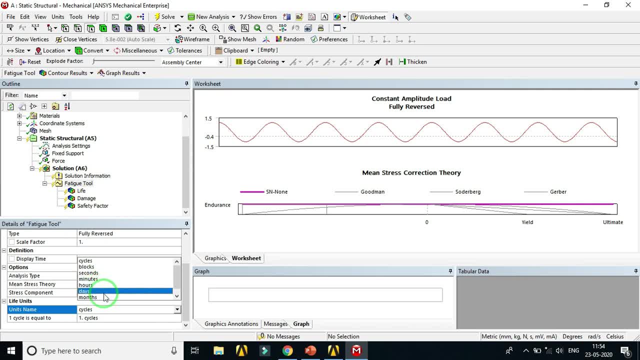 to blocks, seconds, minutes, hours, days and months, So, as per your convenience, you can change these unit types. Whatever type unit you want, you can change it from it. Then one cycle is equal to one cycle, right? So this is. the settings are found in fatigue. 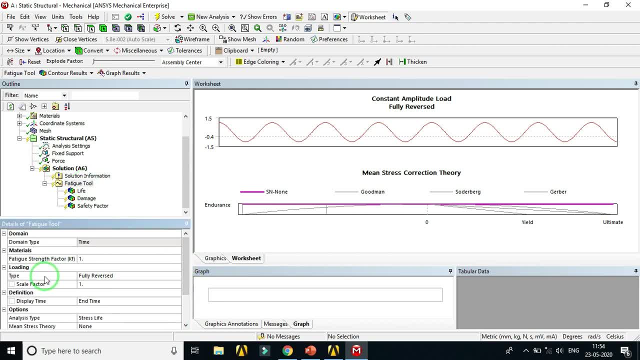 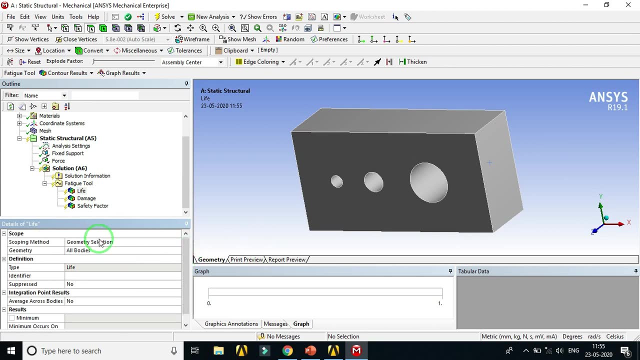 tool. So here the important one is type that is fully reverse. and second is your approach, that is stress life approach. So click on this life. So here we are going to find the number of cycle of this component. Then it is after calculating this life, it will show the minimum life of the component. 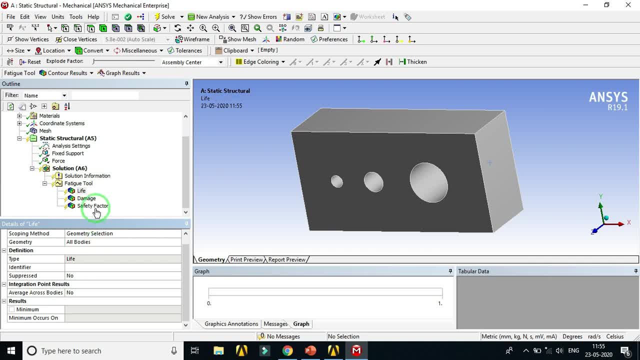 in the particular region, or more stress region. Then second is damage, So in the damage. so life, the design. life is 1 e raise to 9 cycles, So it is very huge cycles. We have given this in the benchmark. and then last is factor of safety. So based on this design factor, design, 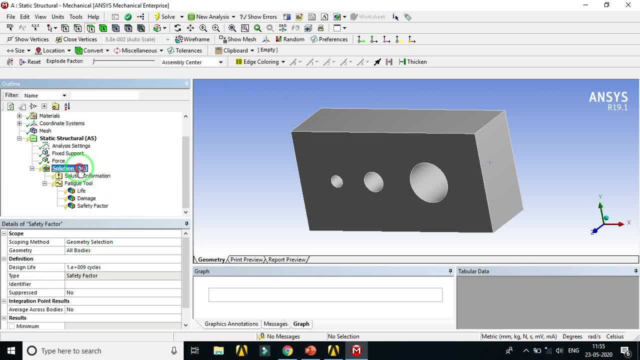 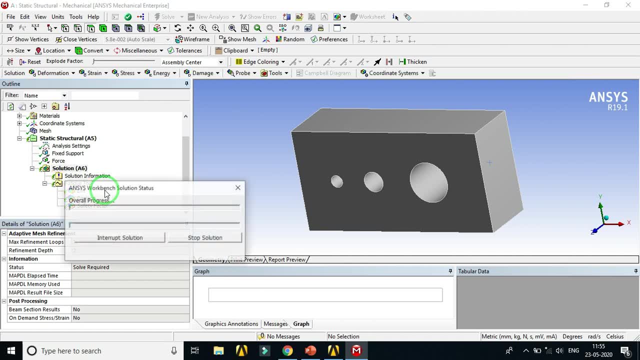 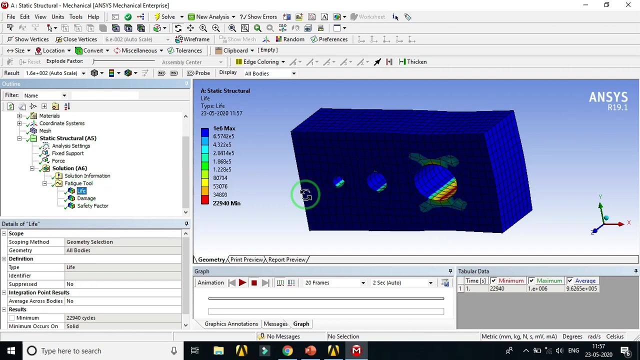 life. We are going to calculate the factor of safety. So solve this. for this, click on right, click on this solution and solve. So solution is ready. So solution is ready Then here, click on this life. So minimum life of this component is 22940 cycles, right. 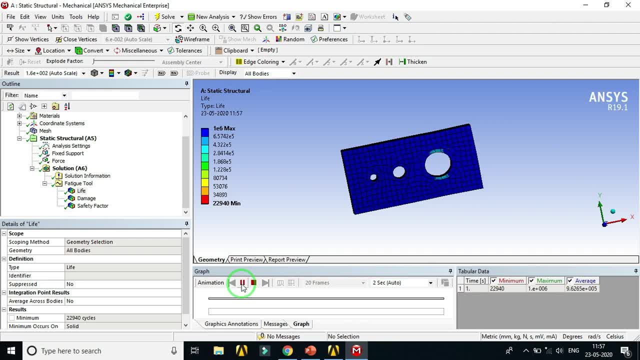 And you can animate this in the animations. Then again click on damage. So here the value of damage is. here you can see in the details of damage the maximum value is 43593 and it is greater than 1 that means the component is going to fail. Why it is so? because our 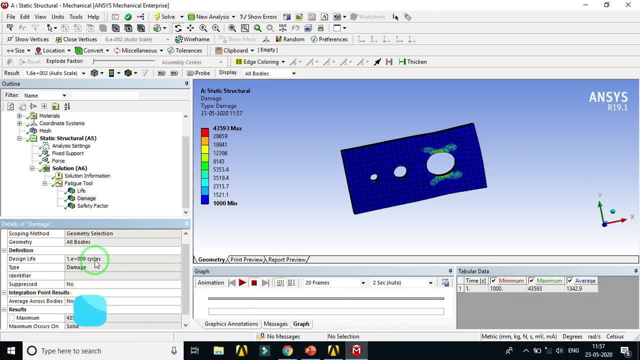 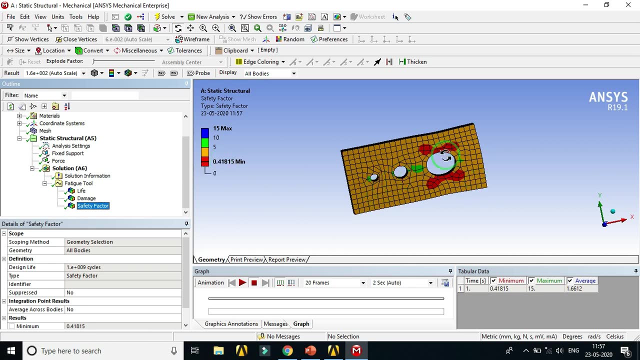 design life is 1, e raise to 9 cycles and it is far less than the values, minimum values, of the component for the given loading condition. Therefore the value is greater than 1 and component is going to fail Again, see the factor of safety. So it is very less than 1. it is 0.41 in this region. So again this: 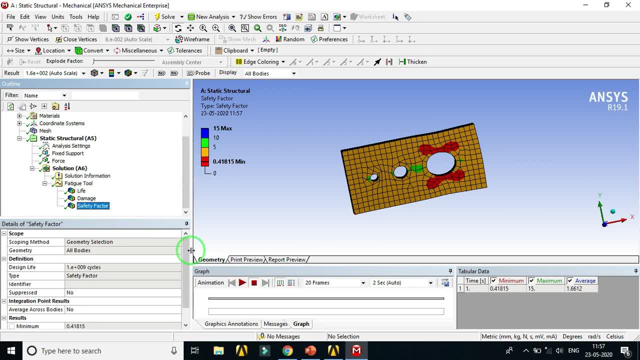 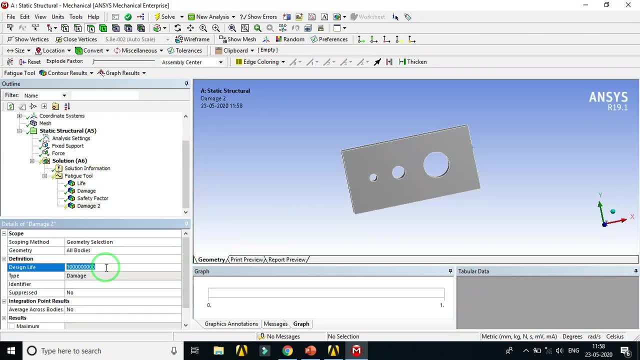 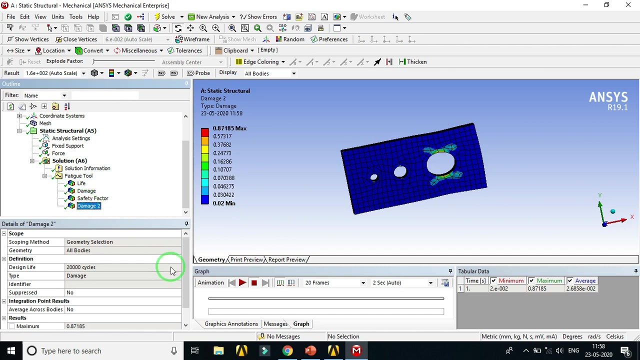 value is again very less. Therefore, suppose I am going to insert again new damage here and for this I am going to change this value to 22, or suppose 20000 cycles is the design life. So here you will find a change After solving when you click on this damage. So here design, 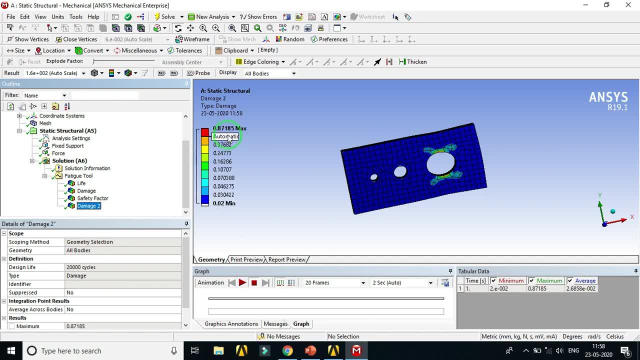 life is 20000 and your damage value is less than 1. it is 0.87 and maximum value is 0.87. that means the value of this design factor is less than 1.. Therefore, for this design life, your component is safe. So this is the purpose of this damage and you are simply. 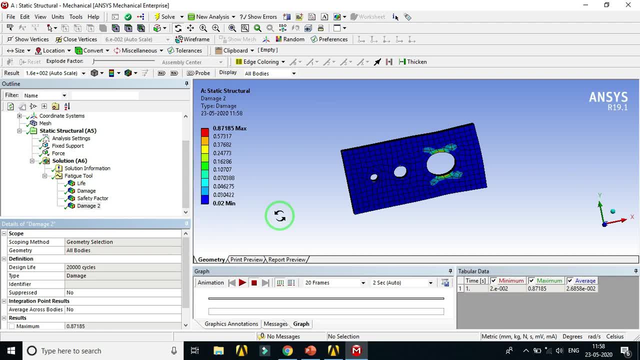 find your component is going to damage or not for the given design life. So it is ratio of design life to minimum life. So your minimum life should be greater than your design life. Therefore, the ratio of this damage will be less than 1 and your component is safe Again. 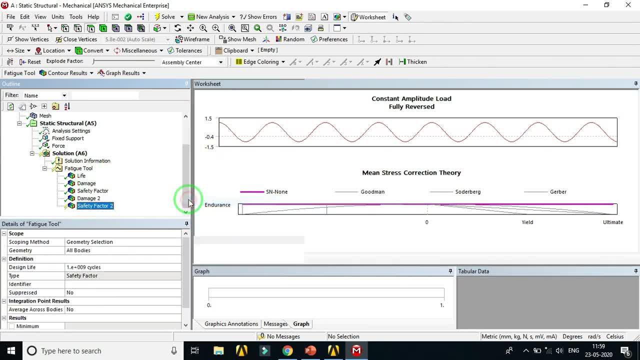 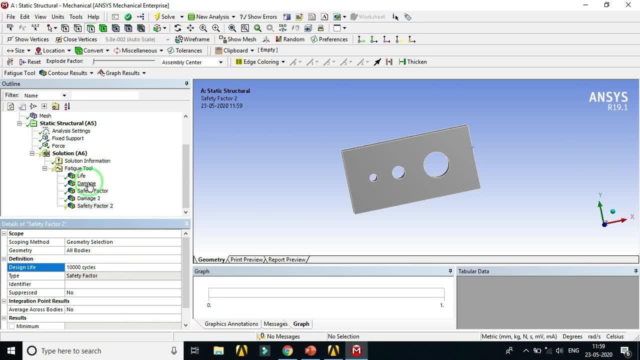 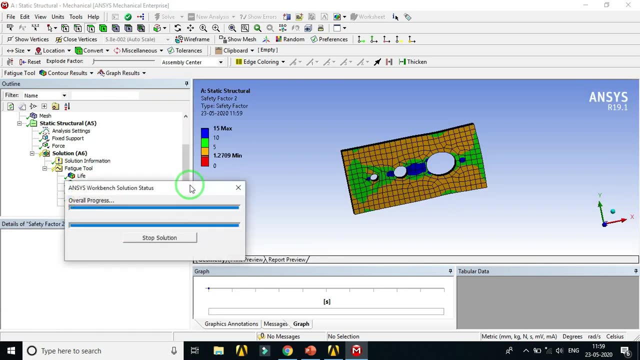 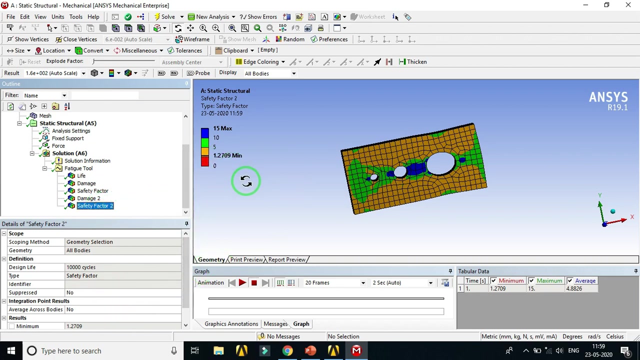 I am going to insert this factor of safety, and here design life is suppose 10000.. So for 10000 cycles again insert For second factor of safety. here the value is 1.27, right, it is more than 1.. So in this: